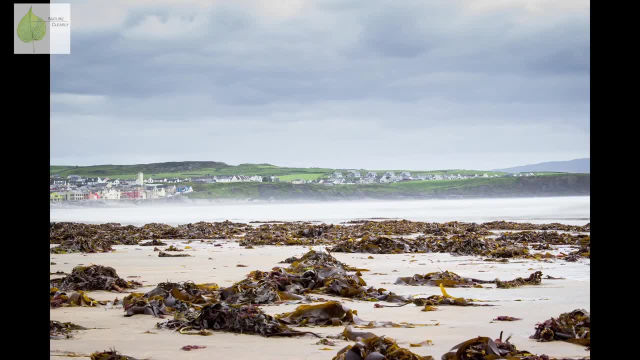 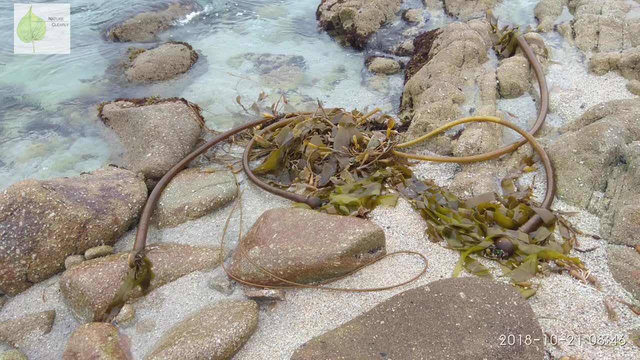 We distinguish three groups: the evolutionarily older brown and red algae and the younger green algae. Even though some species look quite plantlike, with blades that look like leaves and hold faths that might remind you of roots, they are technically not plants. 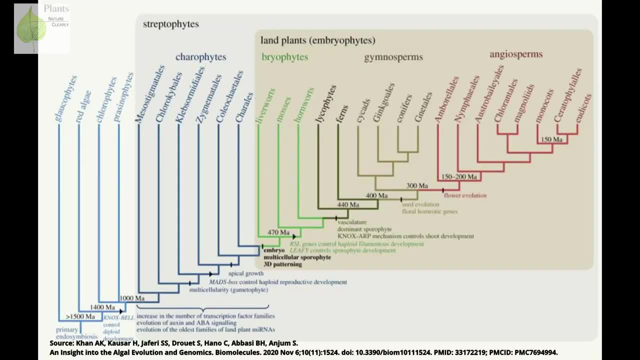 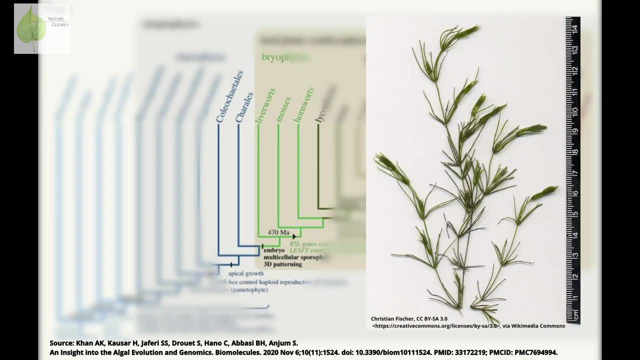 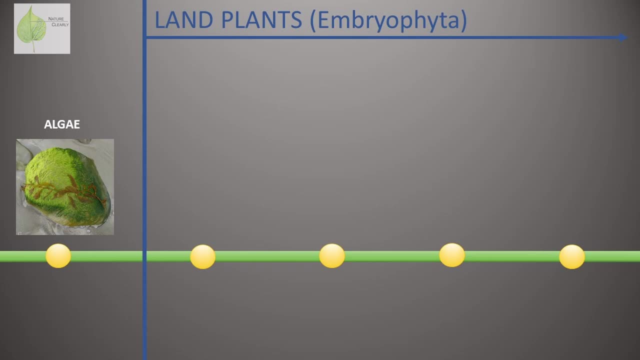 But they are important for our story because, it's believed, the true plants share a common ancestor with green algae, specifically the order Chorales, the stone words. So from green algae we've finally arrived to the true plants. Let's look at how we classify them. 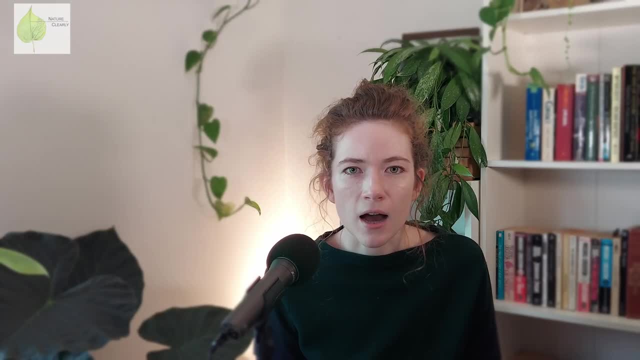 B Land plants or the embryo of a plant, B Plant structure or a plant structure of an egg name name place place, cell location place, etc. or the embryophyta are traditionally divided into four groups: The oldest group, which evolved 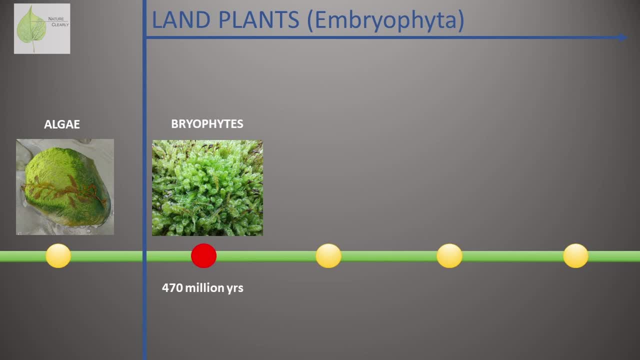 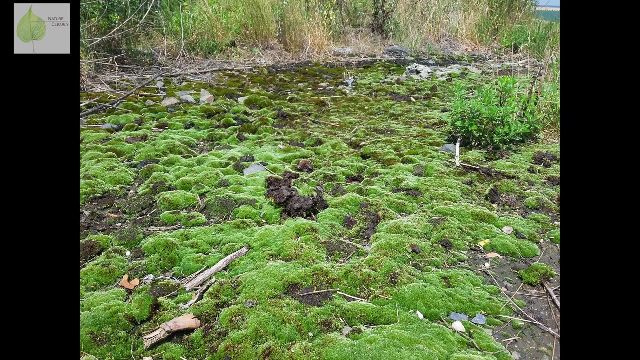 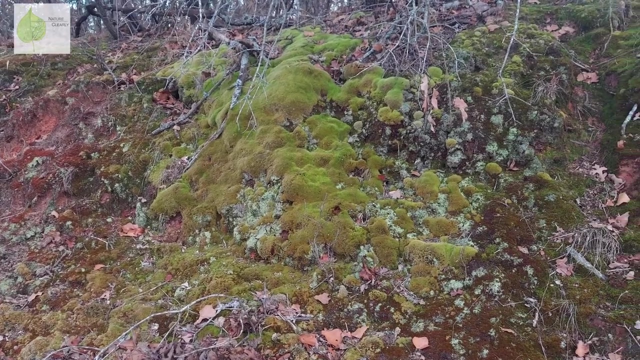 some 470 million years ago, are the bryophytes. Bryophytes consist of mosses, liverworts and hornworts. They tend to grow in moist habitats, although they are not limited to them. Different types of bryophytes often grow together, as seen on this slope covered in different species of 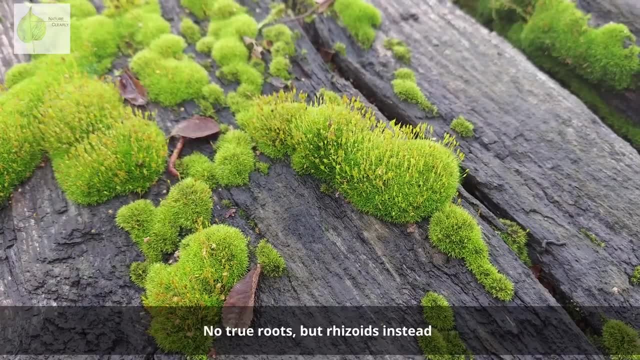 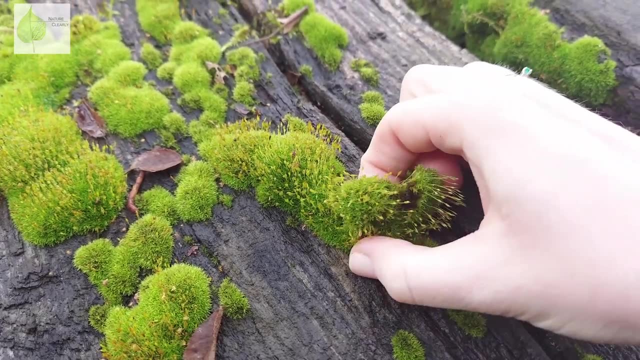 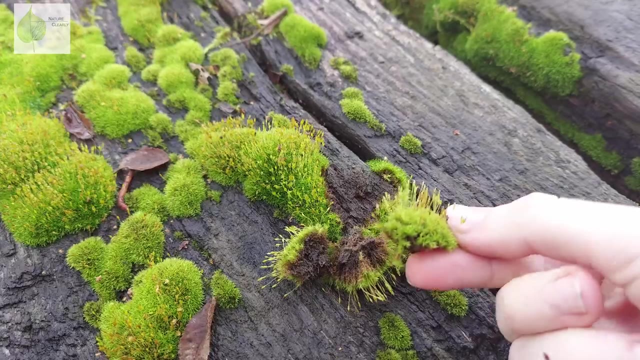 mosses and liverworts. They lack roots and instead are anchored to surfaces by fibrous rhizoids. This enables them to occupy habitats where plants with true roots cannot grow. so you can find bryophytes growing on roofs, rocks and other surfaces without soil. Their 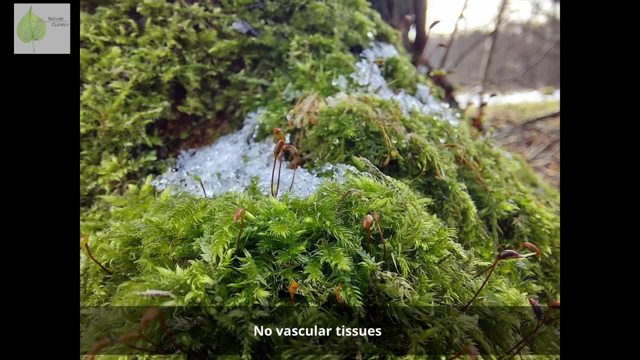 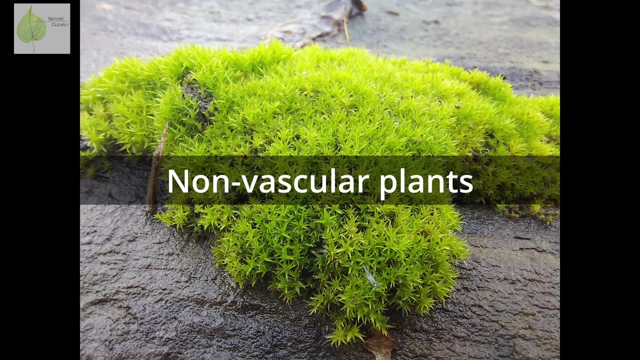 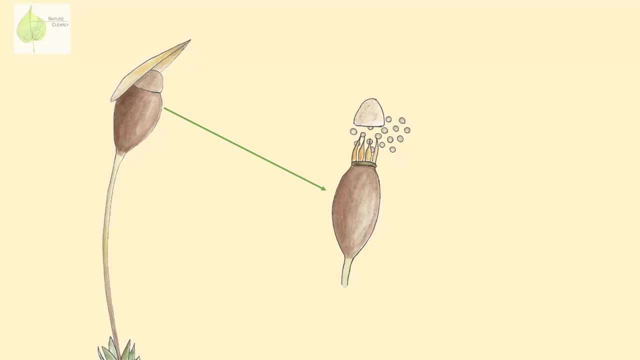 size is limited by an absence of vascular tissues which conduct water and nutrients in plant bodies. For this reason we call them non-vascular plants. You'll also be unsuccessful in finding any flowers, fruits or seeds on bryophytes, Even though they can. 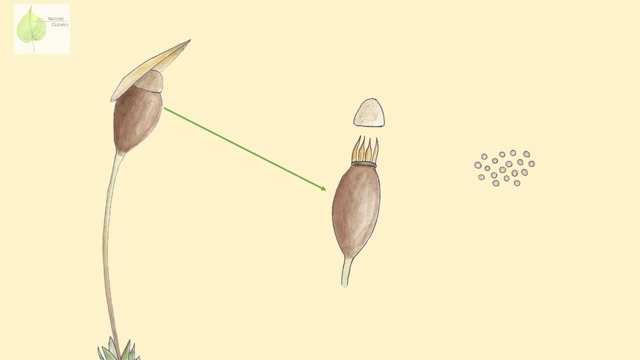 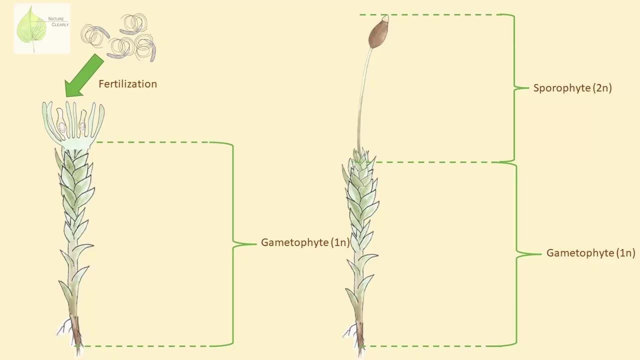 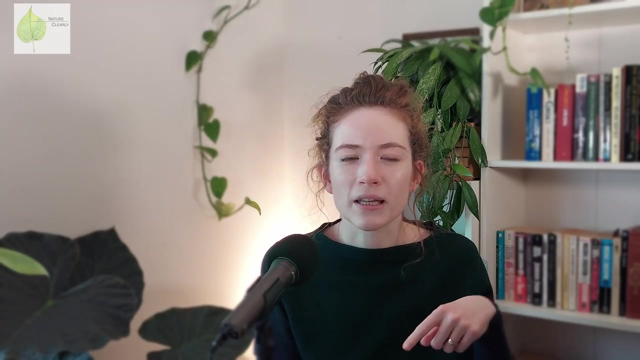 reproduce sexually, they do so by spores. You can actually often see spore capsules on mosses. They look like antennae sticking out of the moss plant. I made a video focused on bryophyte life cycle where I explain all the details. you can watch it by clicking here, and I'll also share the link in. 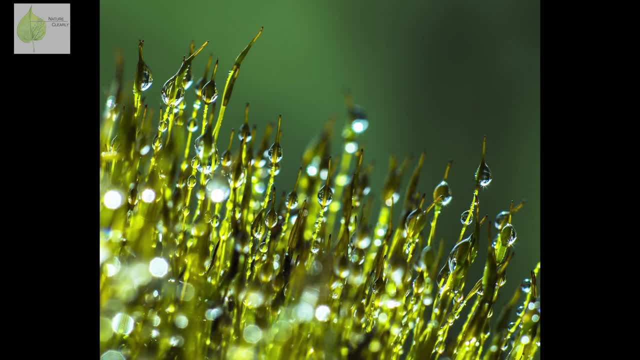 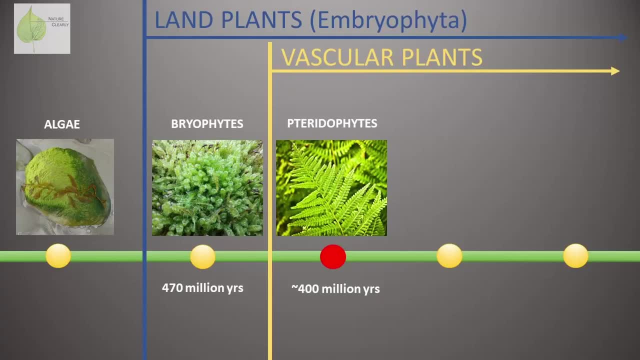 the description below. It's also important to note that bryophytes are dependent on water for their reproduction, as the sperm reaches the egg through water droplets. Going forward with our groupings, all the rest of our land plants have vascular tissues. 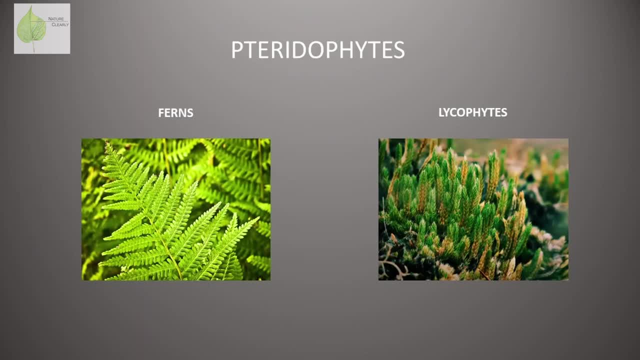 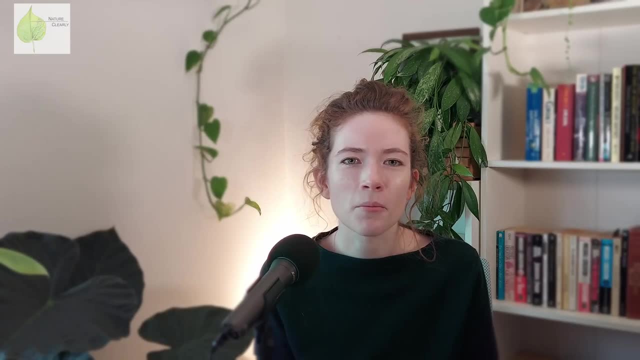 We call them vascular plants. Pteridophytes are the group to which ferns and lycophytes belong. You might be less familiar with lycophytes. Their members are commonly called clubmosses, spikemosses. 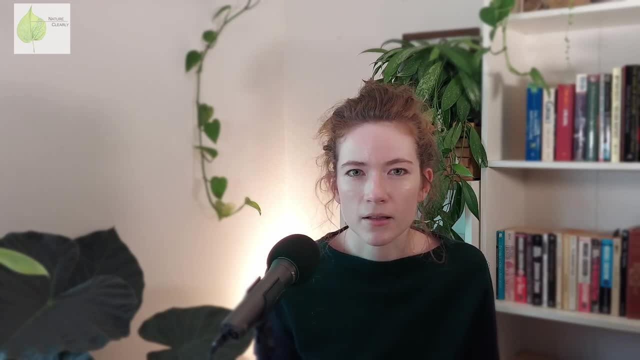 and quillworts, so maybe these terms will ring a bell. To give you an idea, one of the genera belonging to spikemosses are the Pteridophytes. To give you an idea, one of the genera belonging to spikemosses are the Pteridophytes. 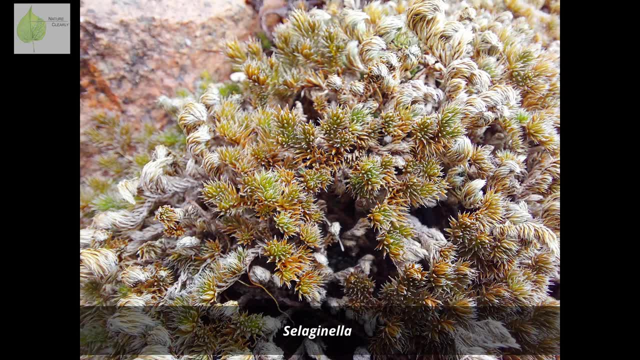 To give you an idea, one of the genera belonging to spikemosses are the Pteridophytes. One of the genera belonging to spikemosses is the widely distributed Celaginella. One of the genera belonging to spikemosses is the widely distributed Celaginella. 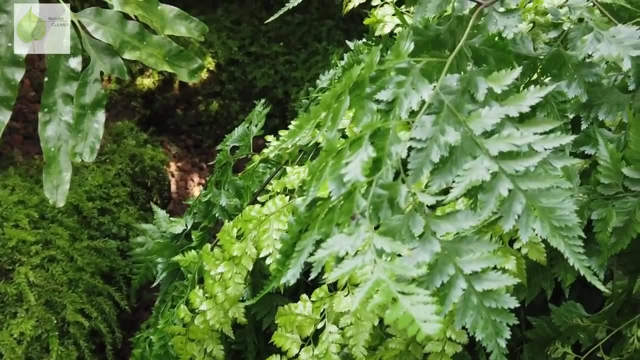 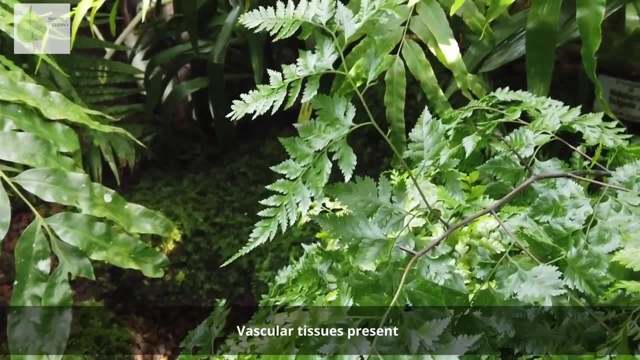 And I probably don't have to introduce you to ferns. Their bodies have clearly recognizable roots, stems and true leaves or fronds. Also, they can grow taller than bryophytes thanks to the presence of vascular tissues. However, Pteridophytes still lack flowers and seeds and, similarly to bryophytes, they reproduce via spores. 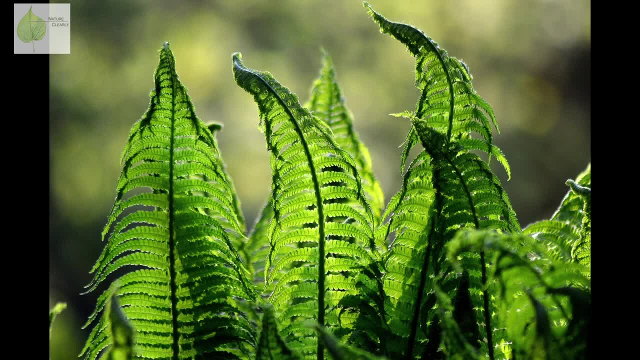 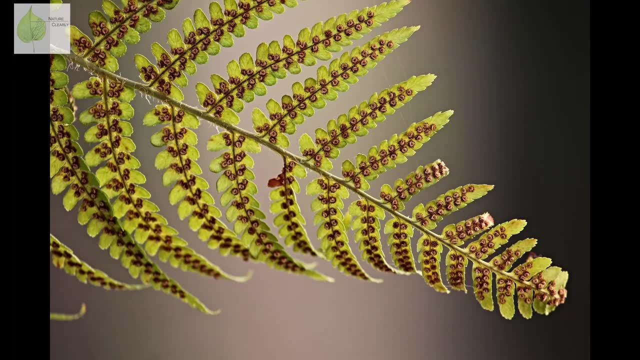 However, Pteridophytes still lack flowers and seeds and, similarly to bryophytes, they reproduce via spores. You might have seen the Sporangia with spores on the underside of fern leaves. They look like little brown blobs. 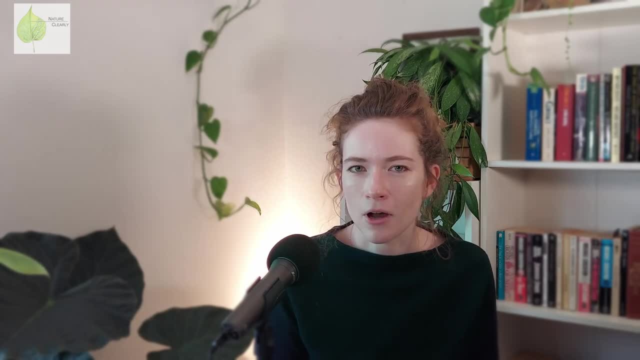 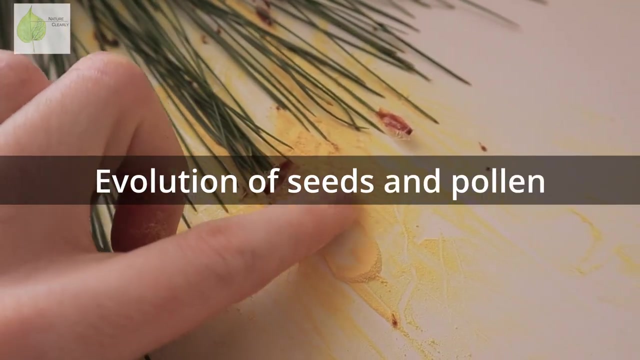 I'm curious to know if you've ever noticed them. Let me know in the comments below. About 350 million years ago, the seed plants first appeared. Production of seeds is a critical feature that brings plants many advantages. Also, the evolution of pollen at this point means that sperm can be transported to eggs. 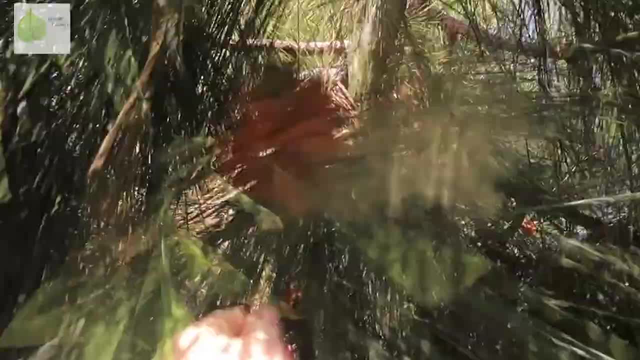 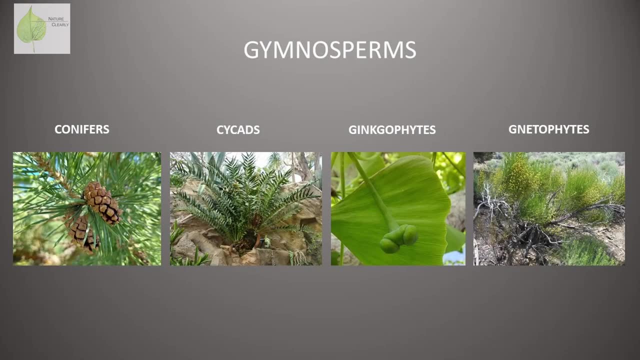 within pollen, grains, by wind or pollinators. Thus, plants that produce pollen do not rely on water for their reproduction. The first group of seed plants are the gymnosperms. Gymnosperms include conifers, cycads, ginkgophytes and gneedophytes. 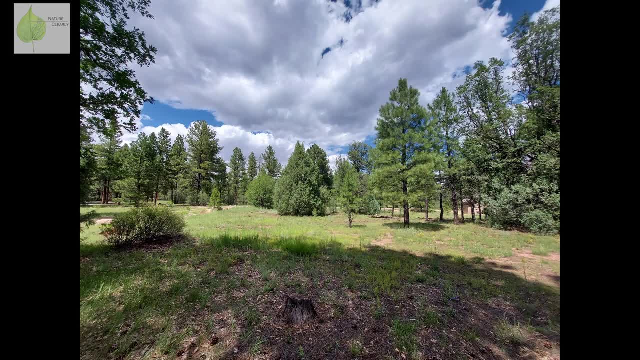 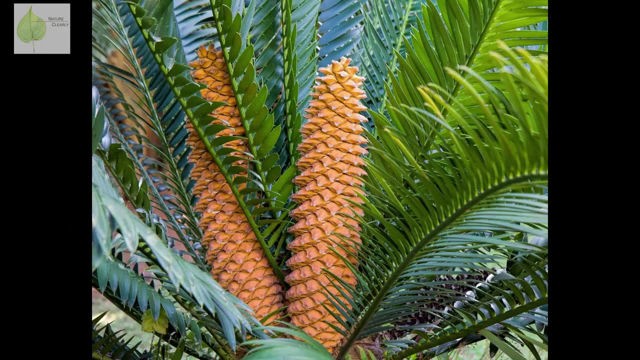 You're all probably familiar with various coniferous trees and ginkgo biloba. the only species in the phylum Gunggophyta is also pretty well known. Cycads are tropical plants that look a lot like palms. 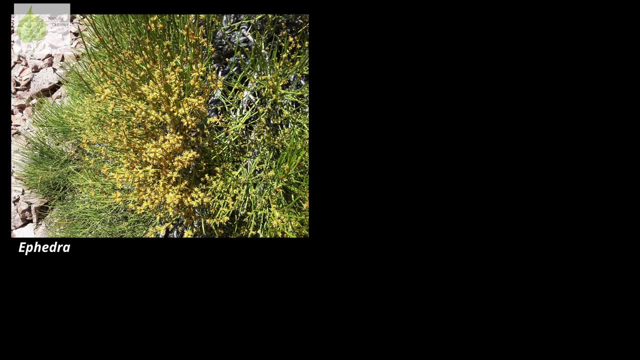 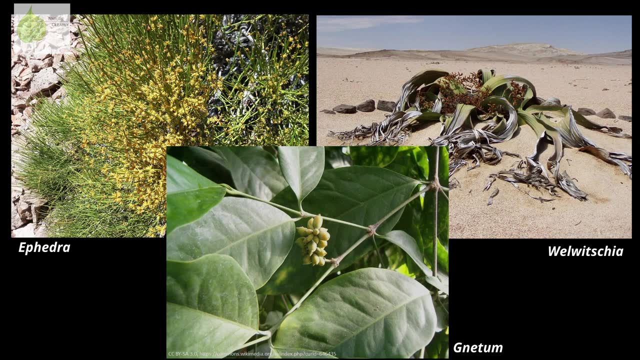 And gneedophytes include three existences. One of them is a very interesting genre – ephedra, the very unusual-looking Velvichia, and gneedom. I think it's fascinating to see these genera that are closely related but look wildly different.